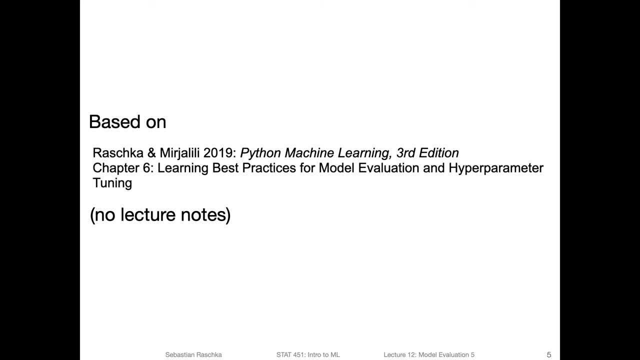 example, making the final exam. The other reason is that I wrote about most of it in the Python machine learning book in chapter six, So I will be sharing chapter six with us on Canvas, which you can use then as reference material for this lecture. Also for this lecture, I think most of the concepts are: 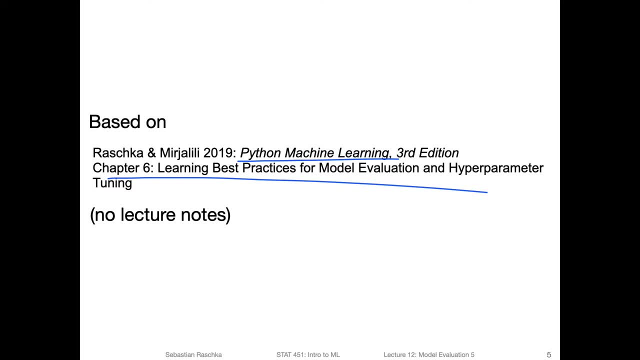 pretty straightforward so that you probably don't need to read up much of it, And so it should be probably all, or most of it should be self explanatory. So the concepts this week are not particularly complicated. So what is the confusion matrix? So 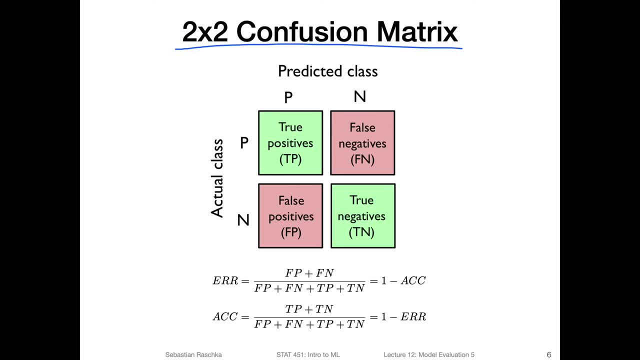 we will start by looking at the classic case of a two by two confusion matrix. Traditionally this was also called contingency matrix. I actually don't know where the word confusion matrix comes from. I mean maybe because it's confusing to take a look at it. 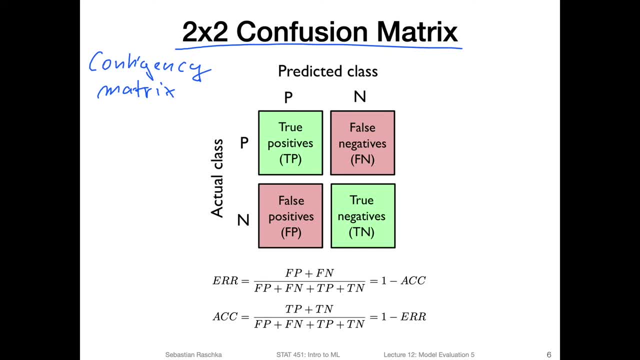 However, I think maybe one of the reasons could be that it's kind of showing us which class labels a machine learning classifier confuses. So what is confusion matrix showing us? it's the actual class labels versus the predicted class labels. So what do I mean by actual class labels? by those I 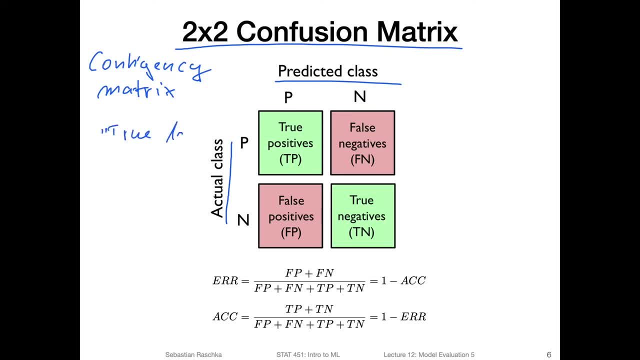 mean: yeah, the true labels in the data set. So now the supervised classification context, or sometimes we also call them the ground truth labels. So these are the true labels in our data set that we want to predict And we compare them to the actual prediction of a classifier. So we look at this: 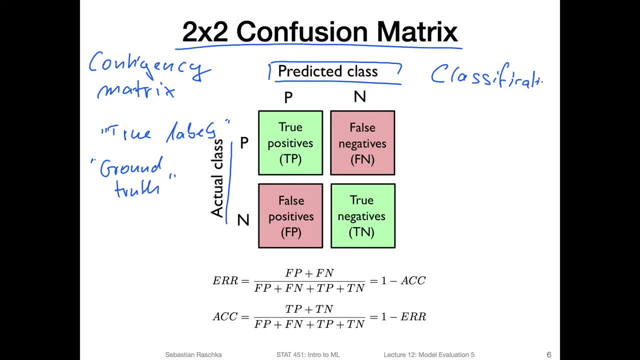 in the concept context of classification And, for example, in a traditional sense, we have usually a positive class. For example, if you think of spam classification, spam is nothing positive. but we could for example say positive class is spam And negative is not spam. 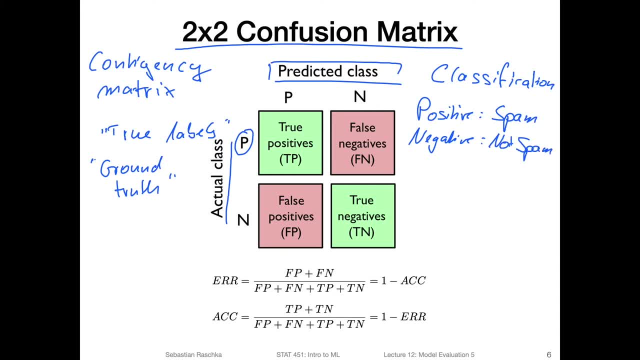 So we have a spam email, a nothing positive in a way that it's not good. However, positive classes, the positive class is usually the class that we want to predict, So class where we have, I would say, stronger focus on. so, if we are concerned with spam classification, we can say: 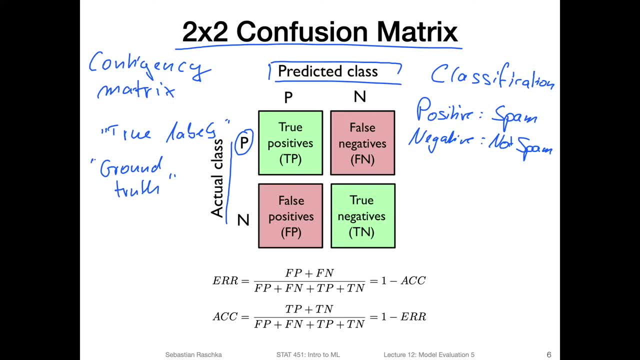 spam is our positive class, And then we can look at the confusion matrix. So here for P, spam it's the actual spam, And here the P means whether we predict, if it's the positive class, whether it's spam. So what I mean is the number of 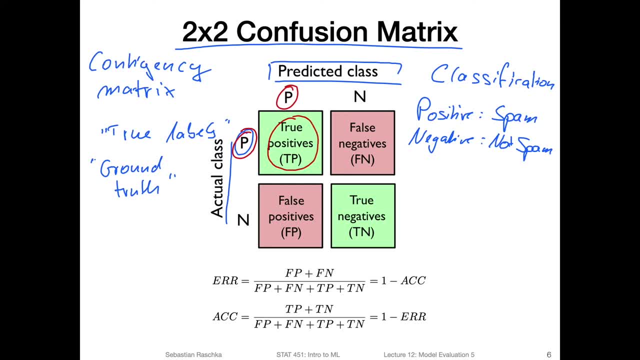 true positives here. true positives mean spam email that were actually correctly identified as spam. So spam identified as spam And the false negatives then this would be: a negative is not spam, right. So a false negative would be then spam email predicted as not spam. So the reason is: so why is? 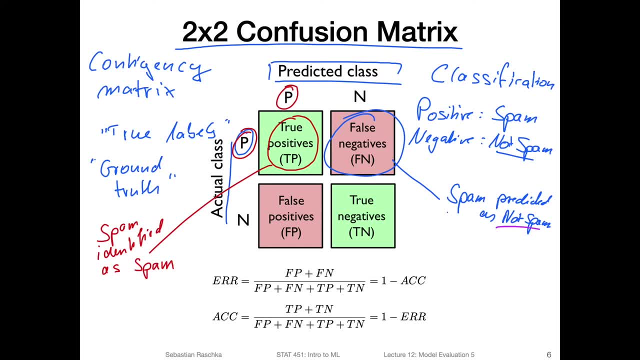 it a false negative. so not spam is here the negative class, but we make a false prediction. So the faults of of this issue. you can think of it as flipping it, So flipping not spam. to the other label: it's spam. So we predict spam as not spam. Then 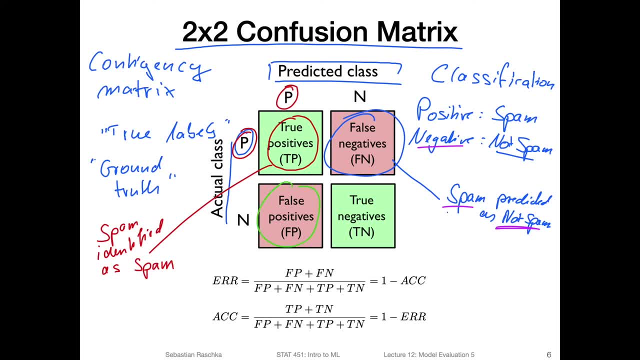 we have the false positives. So what are the false positives? So, the false positives are the not spams predicted as spam And then the true negatives. the remaining part, it's the not spam email correctly predicted as not spam. So yeah, and the ones where we make correct predictions. these 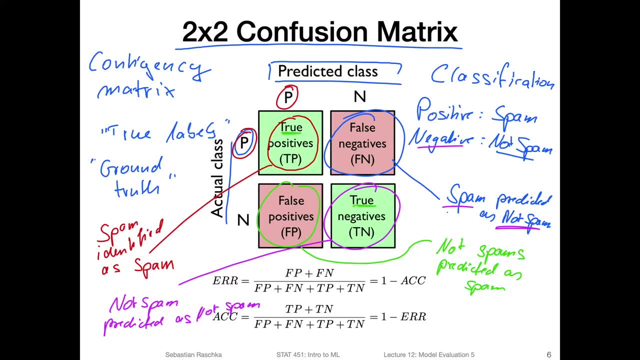 are the true ones, either the true negatives or the true positives, And from those we can also then predict or compute the classification error and the classification accuracy. So for example, when we compute the classification accuracy, we look at the correct predictions and, divided by the 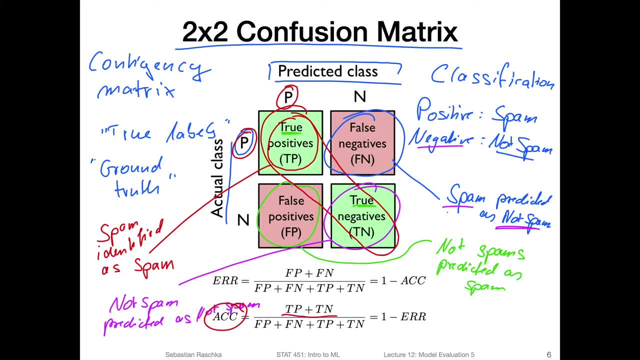 number of total predictions. So we compute the correct predictions, the true positives and true negatives, and divided by all all the data points here, this is like the sum of all the data points, And then from that we can compute the error as one. 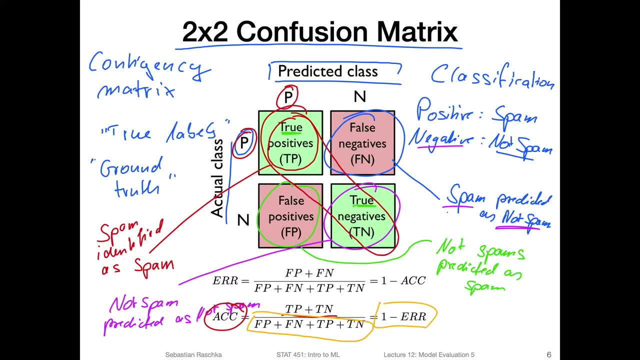 minus the accuracy, or vice versa. we can take a look at the wrong predictions. So we can take a look at these wrong predictions And divide this by the total number of predictions And this gives us the classification error. So in that way, the error. 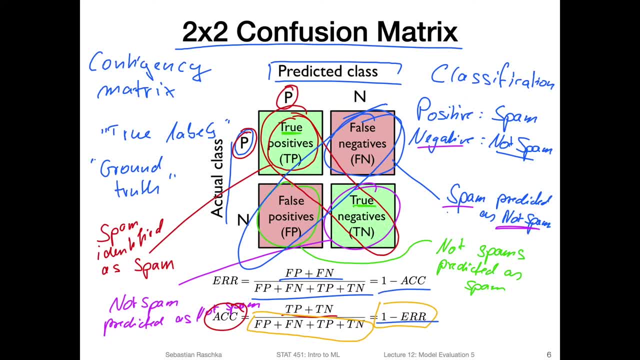 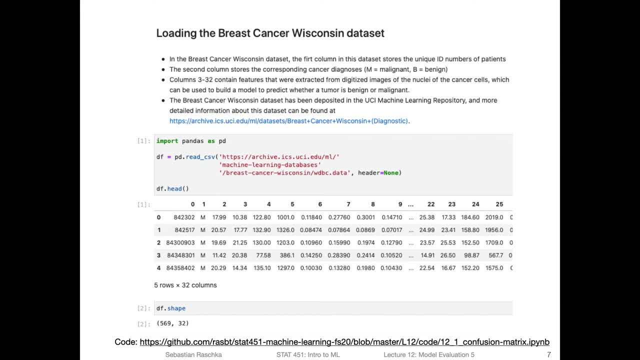 is one minus the accuracy and the accuracy is one minus the error. So this is like the basic concept of a confusion matrix. Yeah, let's now see how we can make a confusion matrix using the tools that we discussed in this class so far, like Python. 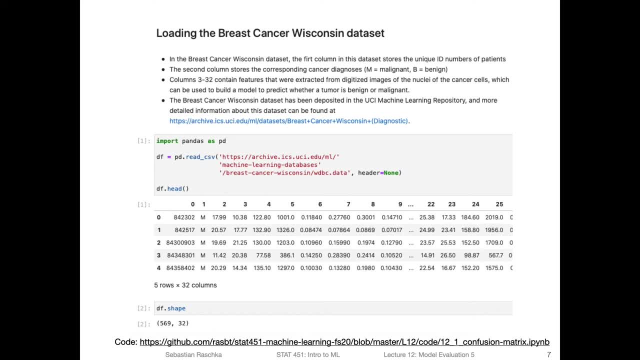 scikit, learn, ml, extend and so forth, And for that we will be working with a new data set. So we will be working with a West cancer Wisconsin data set, So a local Wisconsin data set here. In that case we have a lot of columns this time. 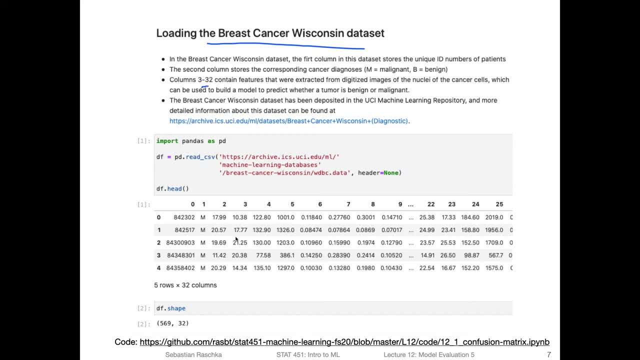 actually up to 32 columns. So what are these columns? the first column- I just see this should be first and not first- The first column- is an ID number for the patient ID. So this first column is the patient ID, And that is some information that is not. 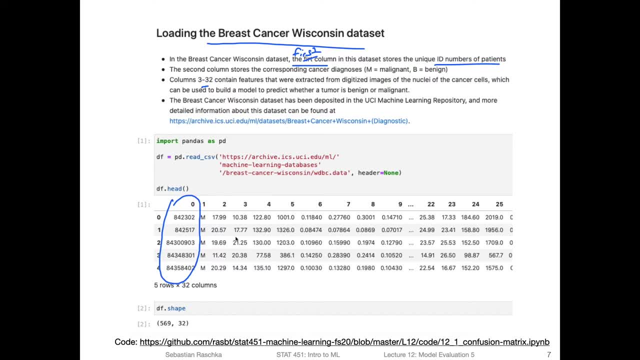 really telling us anything about the cancer. So this is something we would, what we would not want to include in our classifier as information. So we will just forget about the ID column here. The second column stores the corresponding on cancer diagnoses. So, for example, 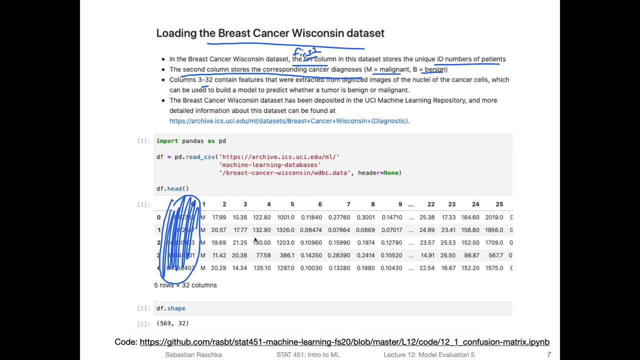 whether a cancer is malignant or benign. these are our class tables, And then the remaining columns- three to 32, contain features that were extracted from digitized images of the AI of the cancer cells, So for those, these are then encoding information about the tumors or cancer, And we can use these for 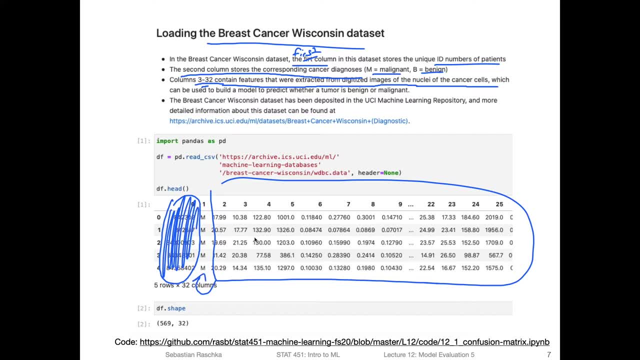 our classifier to predict whether the cancer is benign or malignant. I should note, this is, for example, a typical example of traditional or conventional machine learning, where there are certain techniques for extracting information. So this is: this includes feature extraction that has been done beforehand so that we have this. 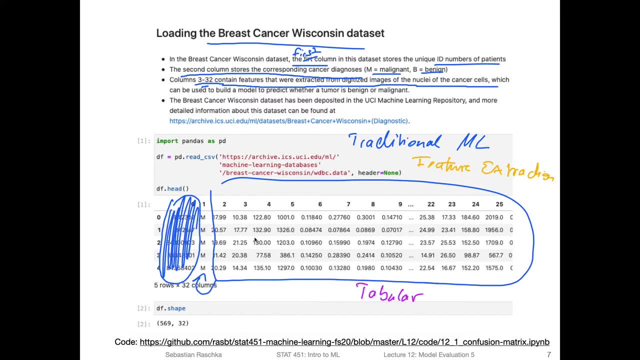 tabular data set. So it's a data set table And the data has been extracted from digitized images. In the context of deep learning, for example, instead of machine learning and deep learning, we would design a neural network. that would also. yeah, that would. 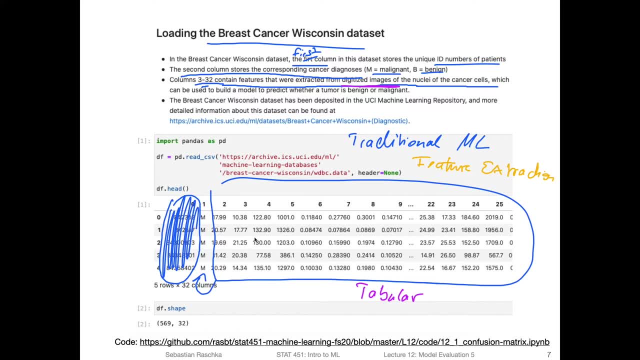 automatically extract these features from the image, So we would feed the images directly to a deep learning classifier. So deep learning is a topic that is covered in stat 453.. And spring where we would, for example, directly feed these image images to the deep learning classifier: The. 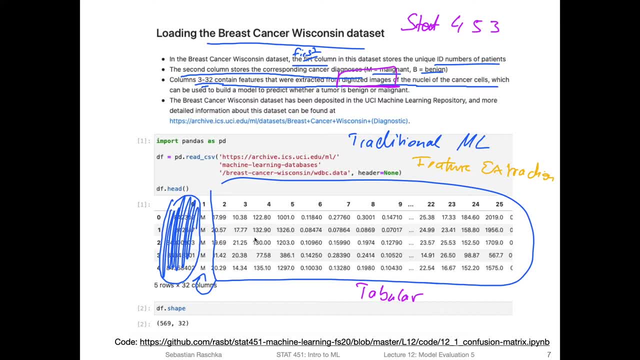 downside of that is that it would require way more data than we may have. So this would usually require 1000s to millions of images to perform or to get a good performance in traditional machine learning, depending on how much you know how much information our features encode. Usually we can. 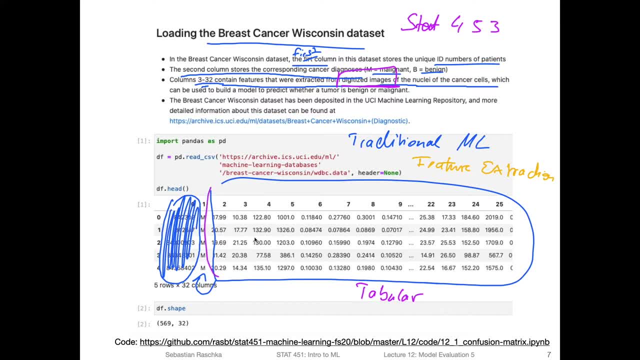 get away with fewer examples, but we have. yeah, we assume the features have already been extracted. Anyways, let's not get distracted by deep learning, but focus on this problem here. So if you want to have also more information about this data set, 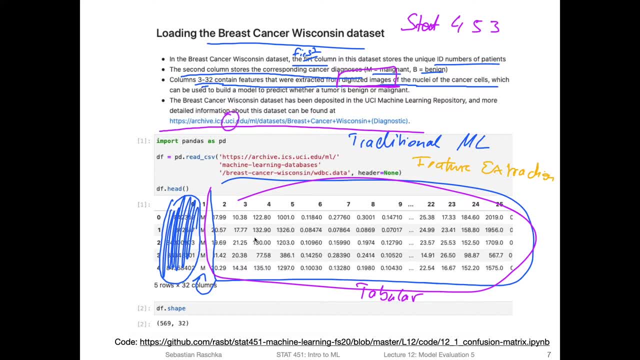 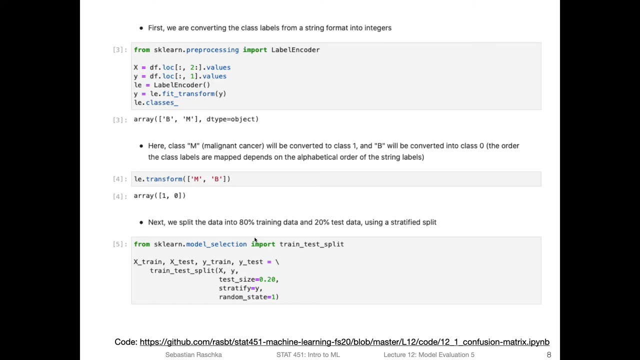 it's also on the UCI machine learning repository. So this is a data repository that contains, or collects, many open source data sets. It's also a good source- Yeah, Finding good benchmark data sets. So what we do first is we convert our class labels, the strings M and B for benign and malignant. 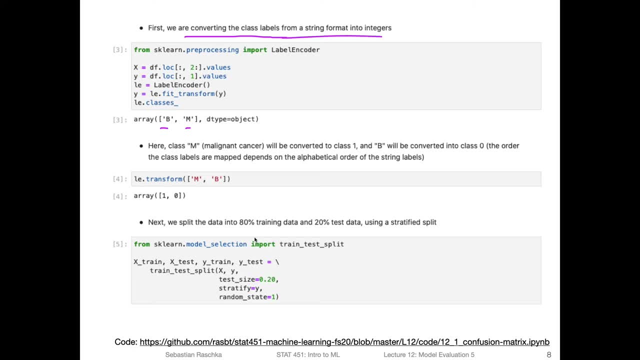 into integer class labels. So we will be using the label encoder from psychic learn and transform these labels. So M will be then encoded as class table one and B will be encoded as class table zero, And usually this is like alphabetically, because B comes from M. So psychic learn does. 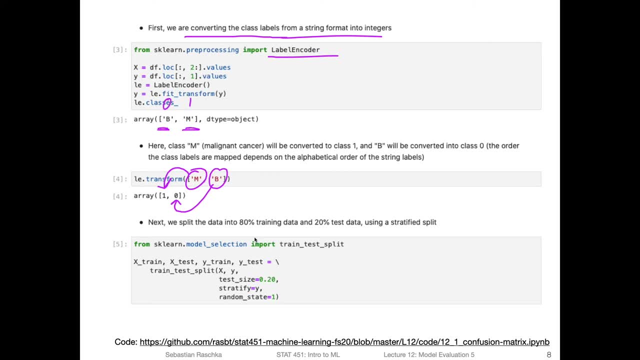 this usually alphabetically. Also, if we don't provide further context, so there will be. we will be looking at precision recall functions later on. we can set a positive label for those. But if we don't specify the positive label, if I go off, 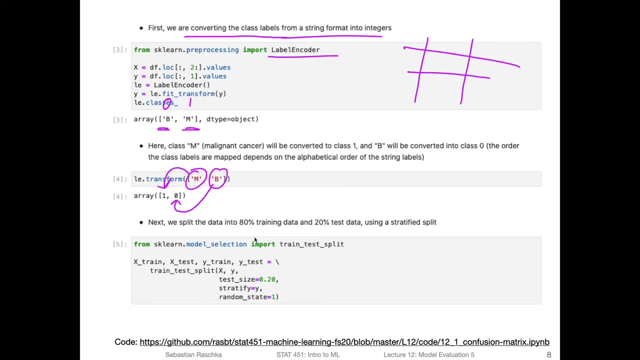 you think back off the confusion matrix where we have the positive classes and then the negative classes by default. in psychic, learn class label. one will be positive, So class level one will be positive, and zero will be the negative by default, However. so now it gets tricky. So my confusion matrix. 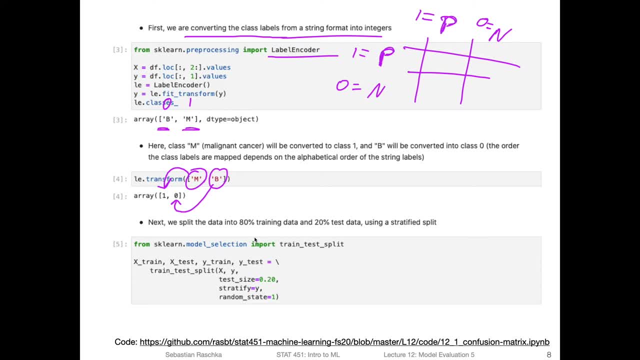 was with positives here. So in this context of psychic learn and ml extend you can. you have to think a little bit differently. you have to think about the class table. it's ordered Even though the one is the positive label in psychic. 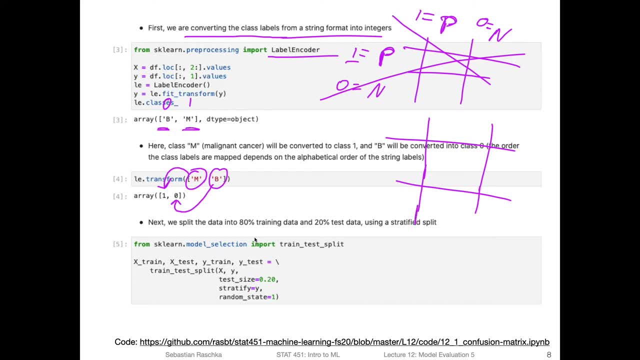 learn and ml extend. it will be numerically ordered, because things are usually ordered. So you will have zero for the negative class here in the confusion matrix And then one for the positive class, like before. but notice that the true positives are now in the lower right corner And the true 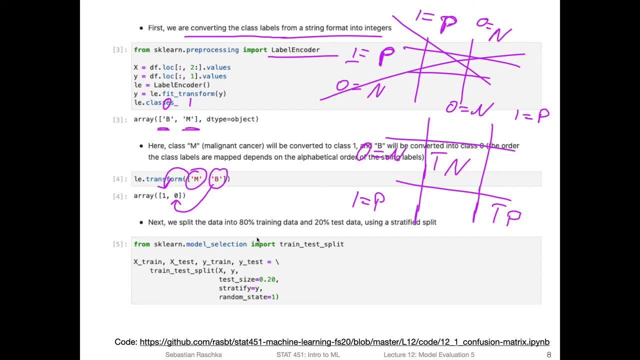 negatives are in the upper left corner. This is usually how we are going to learn psychic. learn on and extend to display these class labels. Why is that? Because we will also see we can extend the concept of a confusion matrix to multiple classes, where 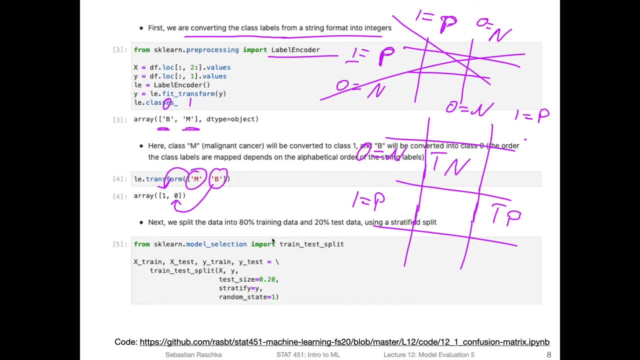 we for example have in the, for example, iris data set case, we have three classes: zero, one and two. So then we don't have positive and negative notions, we have just zero, one and two, And then everything is nicely ordered. Okay, anyway, so it's. 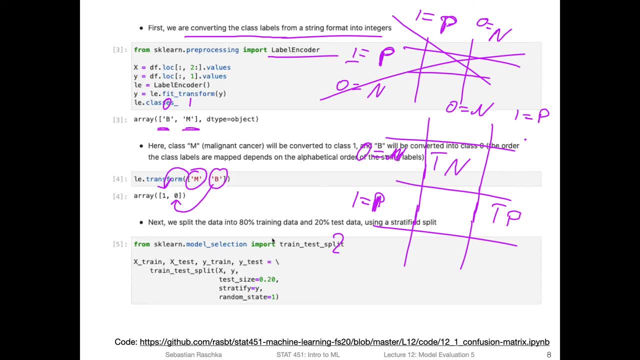 maybe too much information at this point. Second, learn and extend confusion. matrices will give you the true positives in the lower right corner and the true negatives in the upper left corner, So everything is ordered by class tables. Okay, so what we then do is we split the data. 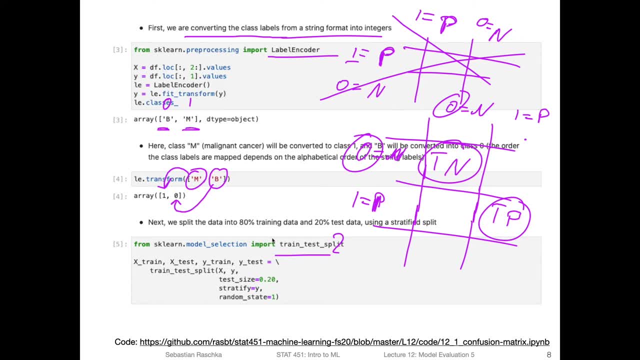 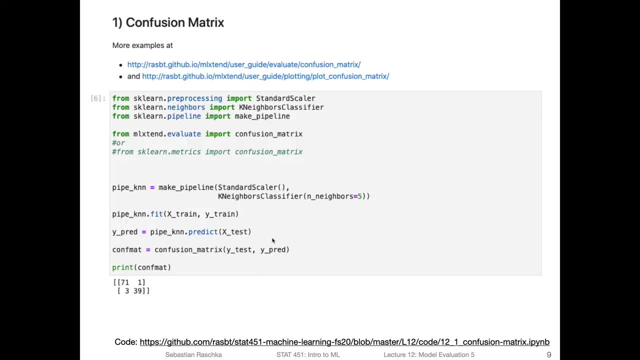 set into a training and a test set. So we have 80% for the training set and 20% for testing. And now we are going to plot the confusion matrix. So here we are going to use k nearest neighbor classifier, As you recall, for k nearest. 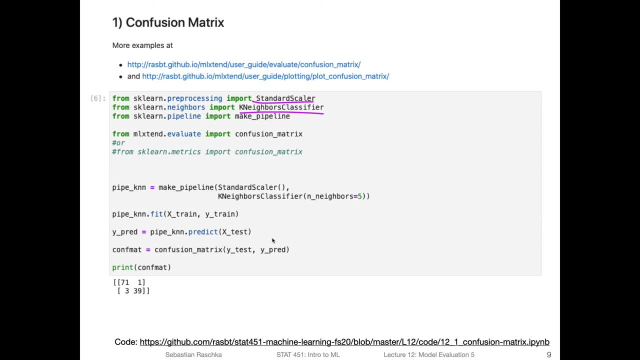 neighbor classifiers. it's important to scale the features, So we also have a standard scalar and we combine them using the pipeline that we talked about before. we will be using the confusion matrix from ml extend instead of second learn, because it has some extra feature that I want to show you. 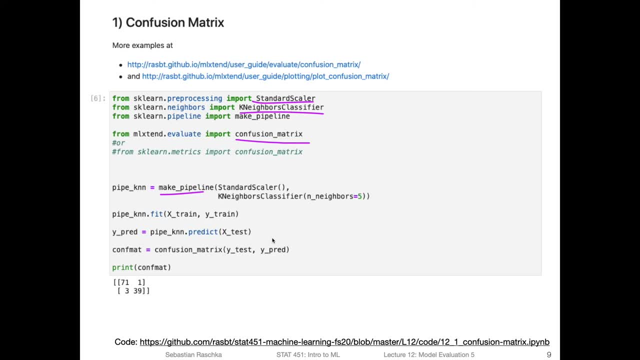 after that. But ultimately, in this data case, they will give you exactly the same results. If you uncomment this one and use the second one instead, you will get the same results. So recall, this is our true positives And this is our true negatives in this case. 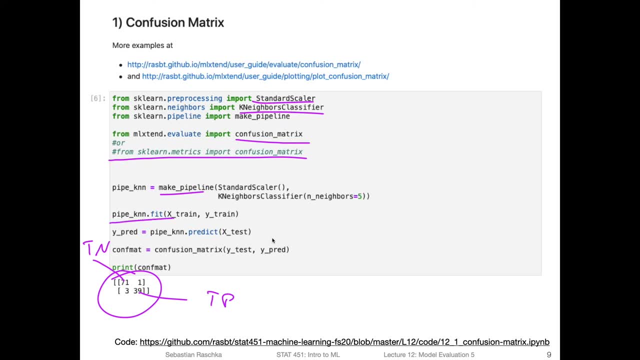 Yeah. so what we're doing here is: we're fitting, we're fitting the k- nearest neighbor classifier, then predicting examples and then calling the confusion matrix on the true labels. So these are true labels And these are predicted labels, And we can see: on the true negatives are in this case,71 And. 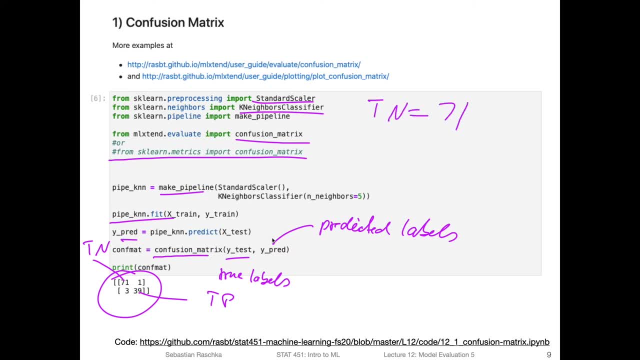 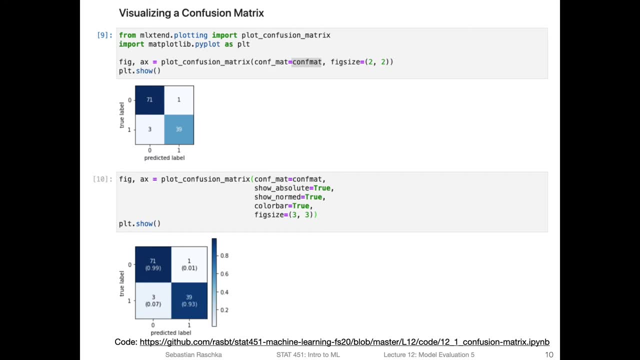 the true positives in this case are 39.. So here is a visualization of that confusion matrix, the array that I showed you in the previous slide using the plot confusion matrix function from ml extent. So this is taking us input the confusion matrix, the array, and visualizes that confusion matrix And that's. 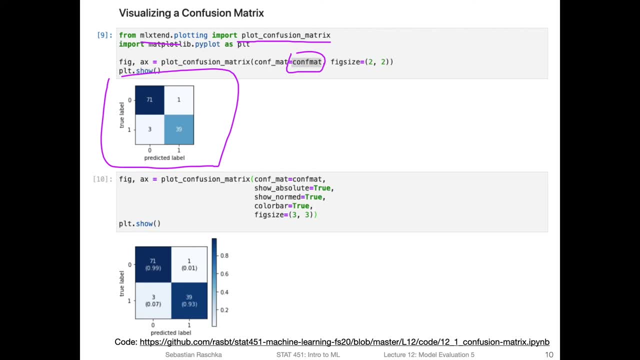 the way is the confusion matrix using matplotlib under the hood. So here, like I said, the class tables will be sorted in ascending order, So the increasing order, so the lowest class table comes first, class table zero and then class table one. here, And if we have, like before, where we have, 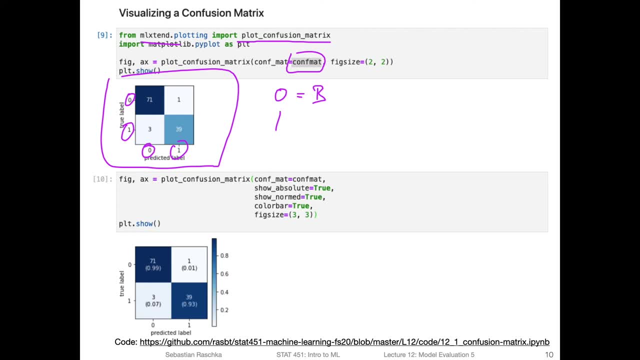 classical zero as benign and classical one as malignant tumor. then we define the malignant tumor as the positive class. I mean this is arbitrary. we can also consider the benign tumor as positive class. It's really application specific. But let's say we go with a convention using classical 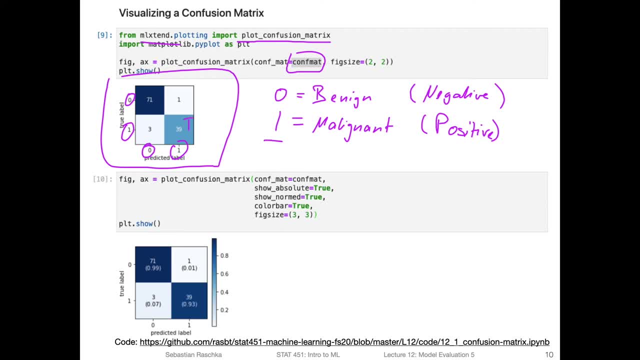 one as the positive class, then this one would be our true positive here, this box and this box would be our true negatives. So there's also a function in ml extends, ml extends confusion matrix function. there's a parameter called show absolute and another parameter short shown. 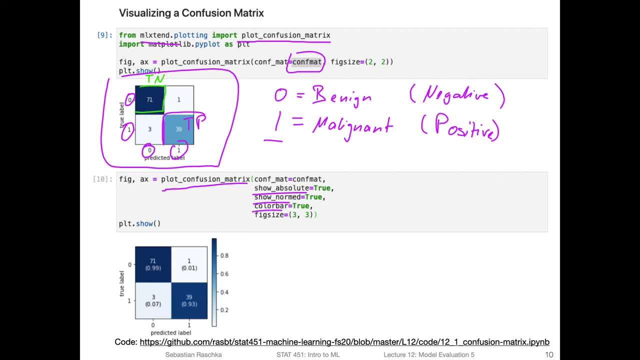 on and another parameter for the color bar. So it gives you some more options. So show absolute. This is by default, true, it shows you the absolute number. So the 39 true positives and 71 true negatives here. So 71 and 39, like before the. 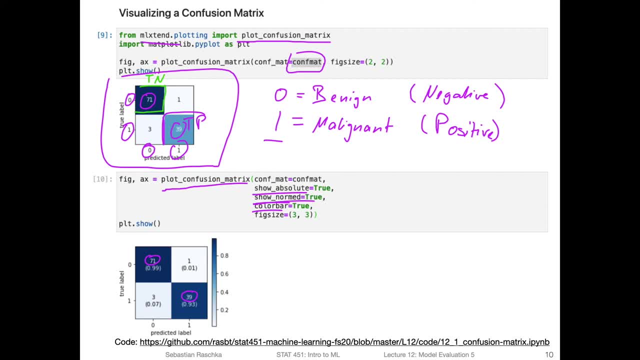 relative one, So the normed one is shown below. This is like normed per row. So what you can see here for the true label, 099% are the true negatives And then 1% are the false positives. So why false positive? because we 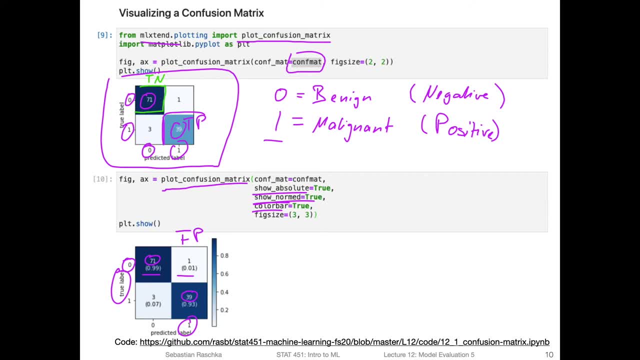 predicted to be positive. However, it's not a positive, So that's a false positive, And this would be the false negatives then. So 7% are false negative for class label one and 93% for the true label, for the positives ones are actually. 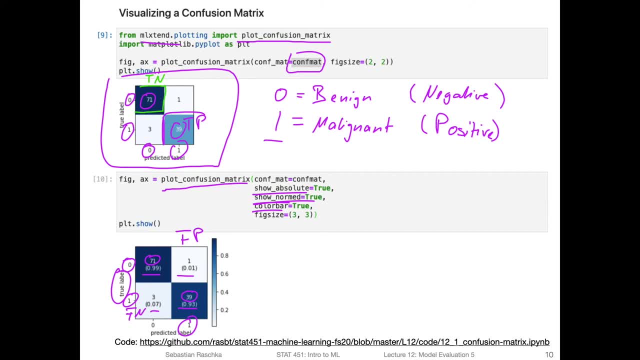 the true positives. So there's just an additional option And then you can also have this color bar here if you like. this can be helpful if you have a larger confusion matrix with multiple classes, more than two classes, And it can be sometimes. 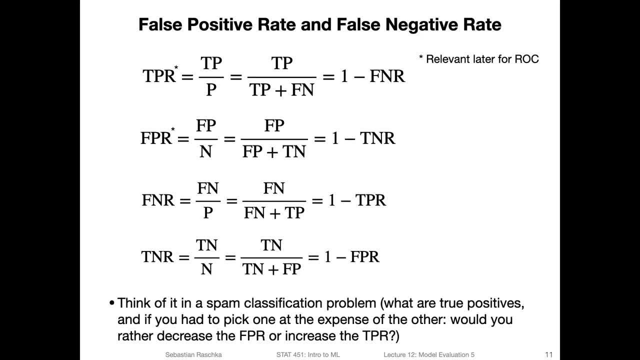 helpful to have a color bar there too. Yes, So now, based on the confusion matrix, we can compute other matrix metrics not matrix. So we have a confusion matrix from which we can compute metrics. So what we have is the true positive rate. 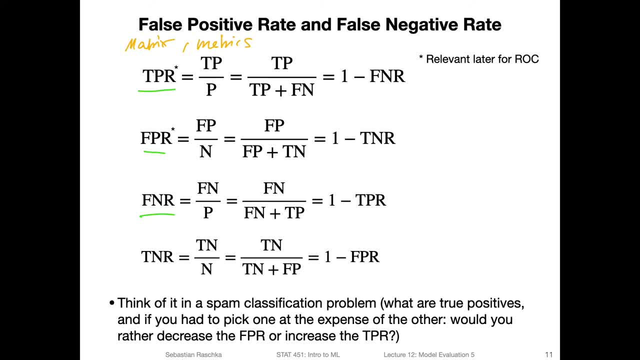 The false positive rate, the false negative rate and true negative rate. why the stars here? that's just to remind myself, to remind you, that these will be relevant later again when we compute or talk about the receiver operator characteristic, which is a very common and popular metric in 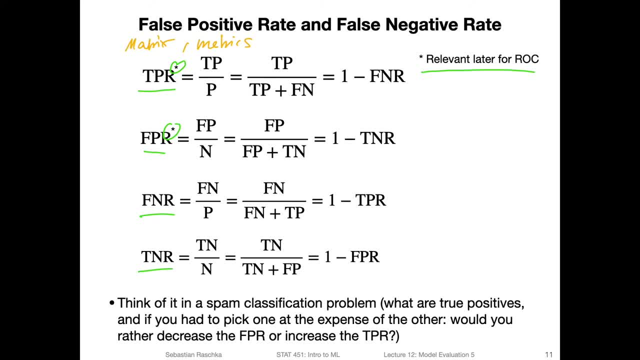 machine learning. So, but now, what we are going to talk about first is, briefly, these true positive rates, just to explain you where that comes from. So let's go back and consider a confusion matrix. Let's say we have the positives and the negatives Here for the, let's. 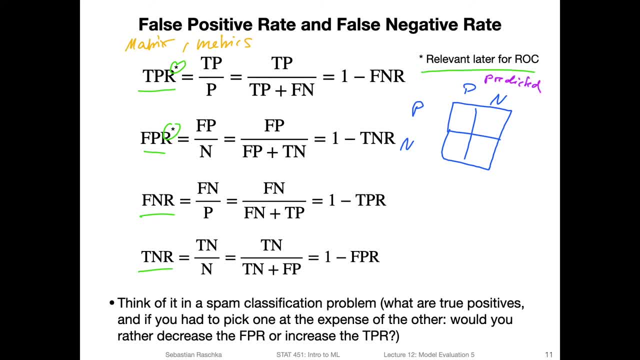 put predicted ones here, predicted positive and negative, and then true or actual- let's call it actual- labels, positive and negative. So yeah, when you think back of the table or confusion matrix we had before, the true positives were here And this here is the number of 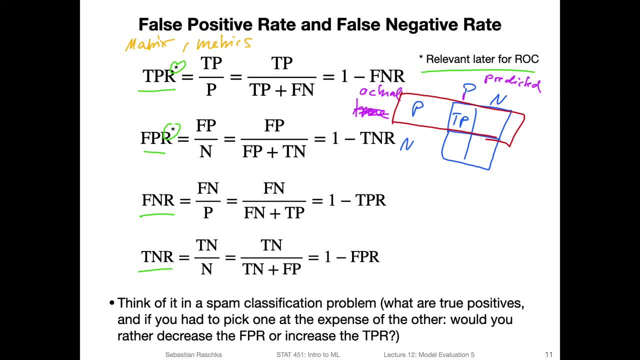 positives. So the number of actual positives can be broken down into the true positives and false negatives. So if we want to compute the true positive rate, for example, we would take this number here, the true positives, and divided by the total number of positives, which is then basically the true. 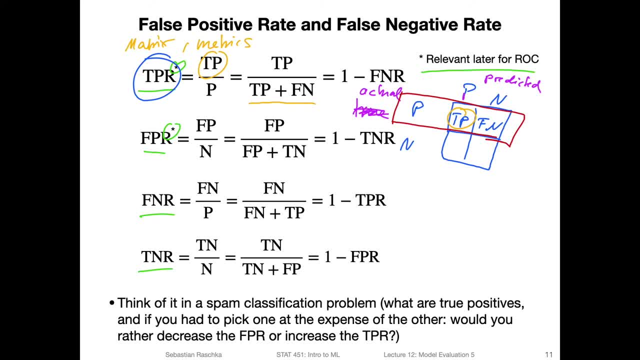 positives plus the false negatives. So if we have, let's say, 100 positives and this value here the true positives are, let's say, 30, then our true positive rate is 30 over 100.. So 33.3%, for example, and we can also 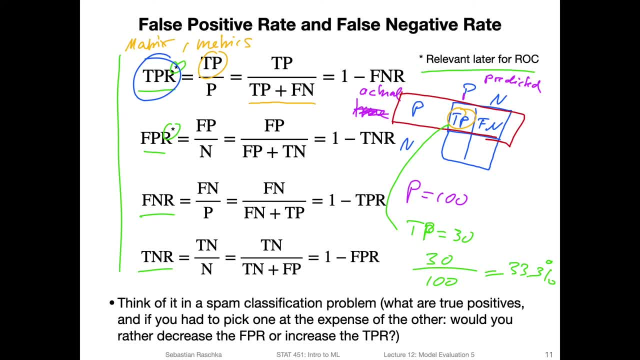 then, using a similar, the similar idea, we can compute these other metrics, metrics So in practice. so what metric do we care most about? I mean, it really depends on the case or the problem at hand. For example, if you think back of our spam classification example, where 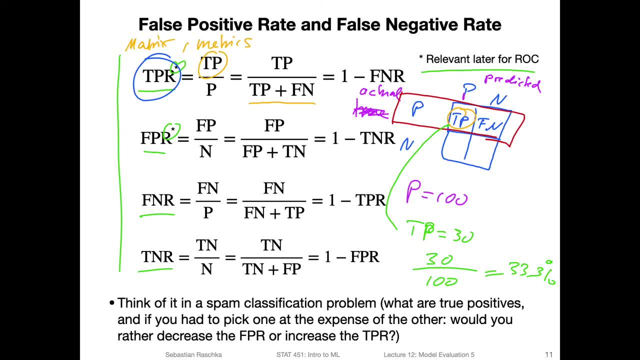 the true positives is like predicting spam as spam. the false positives was like predicting non spam as spam. false negatives would be then spam as non spam, and true negatives would be non spam as non spam. So, what is more, What is something we would be mostly interested in? So I would say: 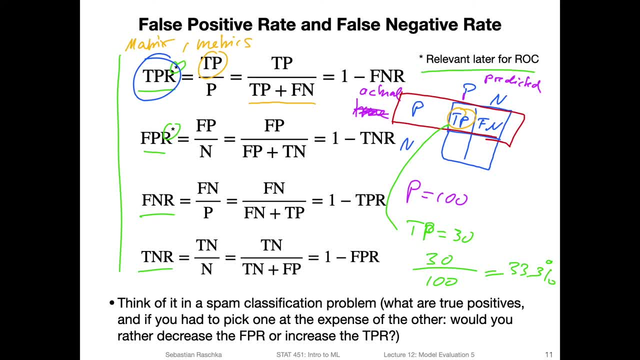 increasing the true positive rate is great. So if we increase the true positive rate, we increase the probability of having predicting spam- if it's actually spam, right. So that's good thing. I think what we really want to avoid, though, in 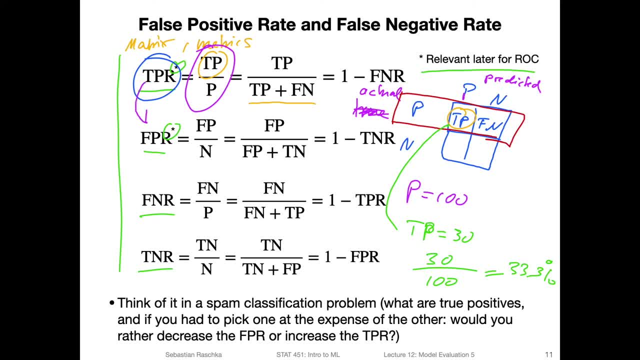 a spam classification example. if we have to pick over true positive and false positive rate- we will later see the true positive and false positive rate We will later see there's like a small relationship between the two, So they're kind of tied together. So if what's more? 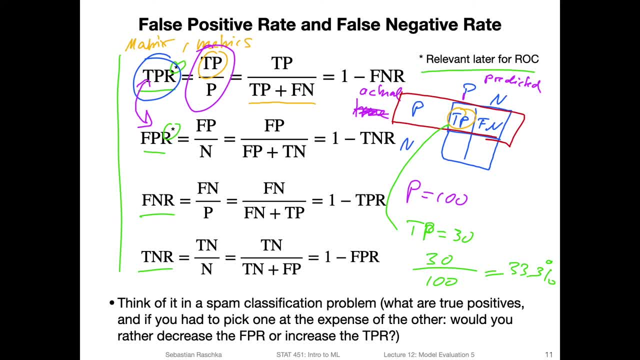 important like improving the true positive rate or decreasing the false positive rate. if I have to pick one over the other, I would maybe, in the spam classification example, emphasize the decrease, decreasing the false positive rate. right, Because if you think back of the false positive, 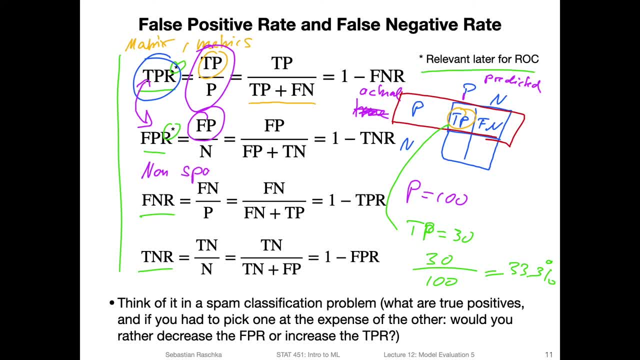 this is non spam classified as spam. and now think about it from a user experience. If you have an email inbox, it can be super annoying if you have spam in your inbox, right? So if you have case where you have spam in your inbox, whether classified didn't. 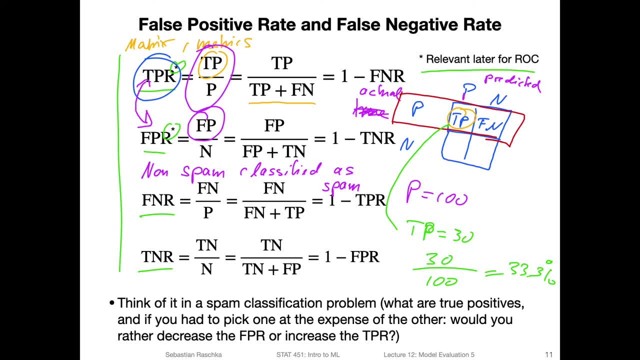 really classify spam as spam. this would be annoying. So if you have a low true positive rate, that would be annoying. So if you have a low true positive rate, that would be annoying because you have a lot of spam in your email inbox. 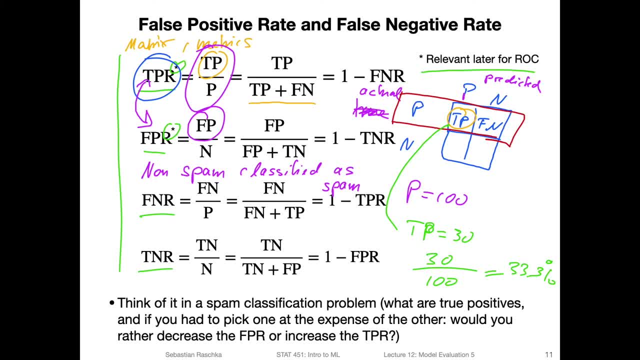 However, it's not the end of the world. you can always click the Delete button. However, how I use my email, I usually almost never look at my spam email. And now imagine you have a high false positive rate. that means the classifier predicts: 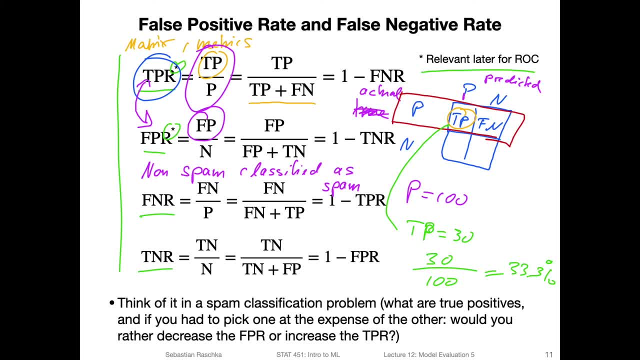 something is a spam, although it's not a spam, So it gets automatically moved to your spam email box And then imagine that's like a very important question, like something about your grade, or you asked me an important question about the exam And I don't get to see it because it's now in the spam. 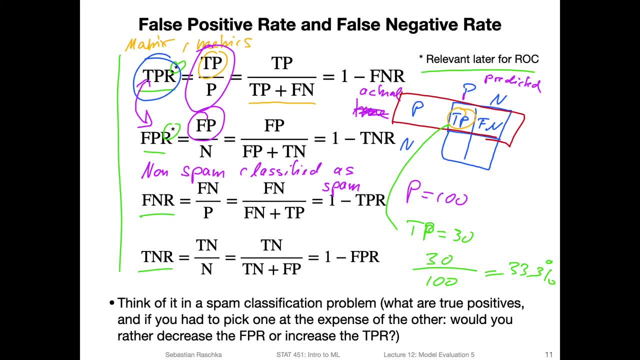 box. So this would be really bad right. So in that way I think in the spam classification example, if I would pick one over the other- I'm maximizing true positive rate or minimizing false positive rate- I would pick minimizing false positive rate and be okay if there are. 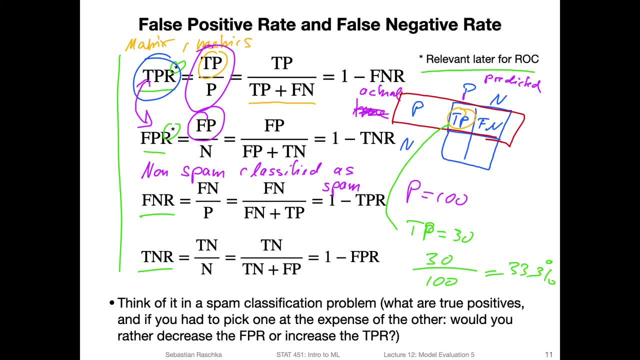 sometimes spam email in my inbox. I can just manually delete them, Of course. ideally we would have a low false positive rate and a high true positive rate, But it's not always possible. So yeah, here's an illustration of that issue. 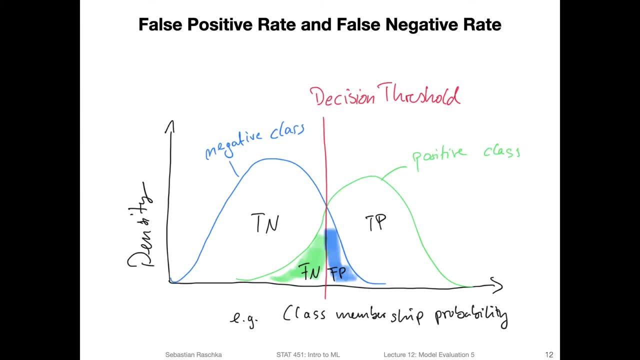 So what I was trying to visualize here is that it's not always possible to have, let's say, zero or false positive rate and very good, true positive rate. So there's usually a trade off. So consider this case. we have one feature And 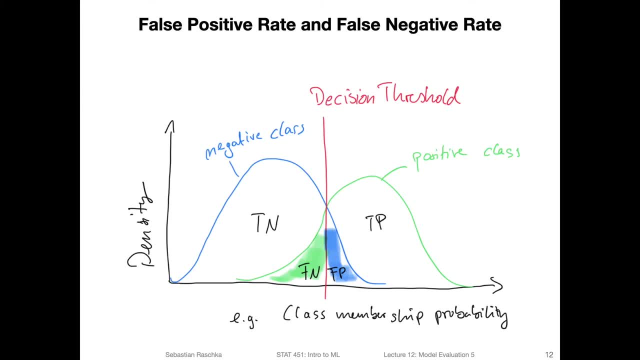 yeah, because we talked about spam. let's continue talking about spam. So let's say, you have some numeric measure what makes a spam and not a spam. So here on the left hand side, the negative class, you have all the spam emails. So we have some numerical feature here for those. 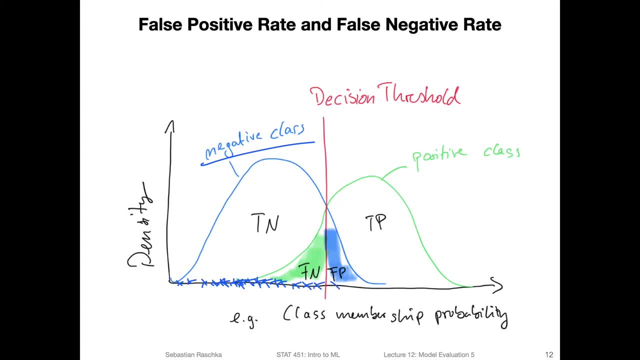 And there's a high density of those in the center And it's basically a distribution of the feature values. you have a lot of examples, So each x here is one training example And here the same for my own spam email. So I have also a lot of spam. 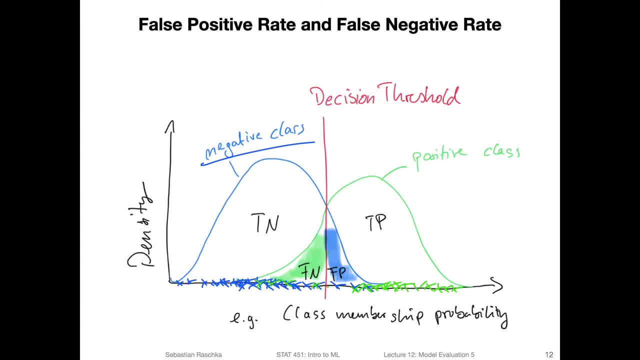 email And it goes up to here. So not that many, But yeah, So here is the density of that. So relatively how many fall into that region for each feature? And you cannot see it's not possible, based on that feature, to make a perfect prediction. 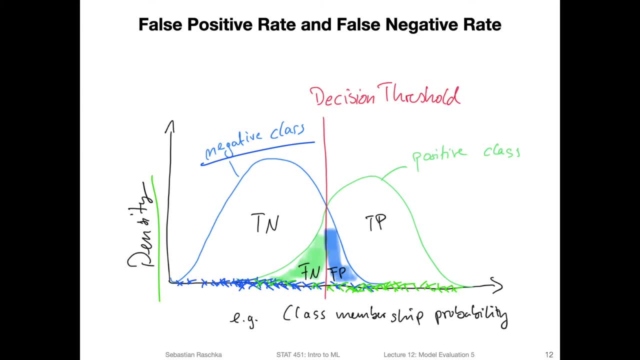 right. So because there's an overlap between non spam and spam, they have, some of them have very, or have similar features in this region here, So it's not possible to distinguish between the two. I have a decision threshold here. this is my decision. 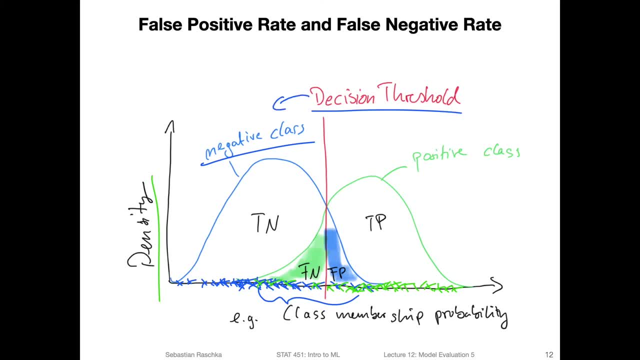 boundary If I say everything left of my decision threshold is predicted as negative and everything right of my decision threshold is predicted as positive as spam. So I will get that correct. a correct prediction most of the time, because you can see the bulk of positive classes here is actually 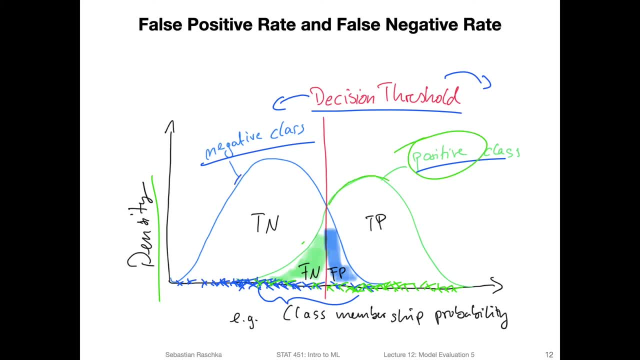 to the right, So there's a high density here And the bulk of the negative class here is to the left. However, I will make some wrong predictions, right. So if I predict everything left from the decision boundary to be non spam, 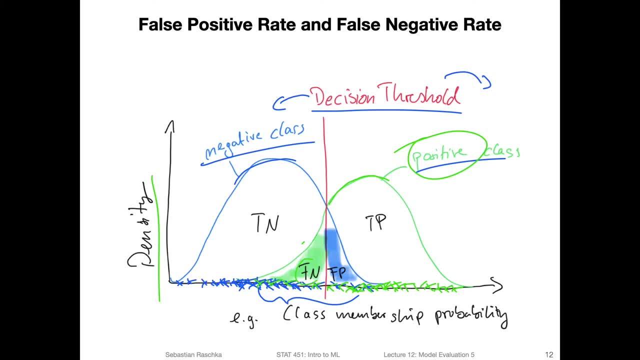 I will actually get those here wrong. These are my false negatives. So I will predict they are negative, but it's actually wrong. They are not negative, they are actually positives. On the other hand, if I predict everything to the right as spam, I will get some false positives. So these here: 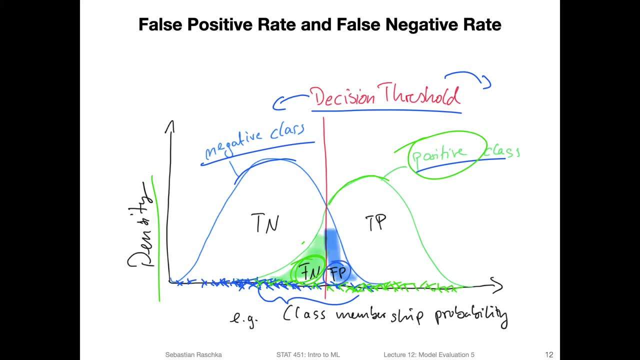 these are the ones that I predict as spam, but they are not spam. And these are the bad ones, right, Because these are the emails that we may miss, because they are important emails and they could be accidentally moved to our spam inbox. So now I can actually. 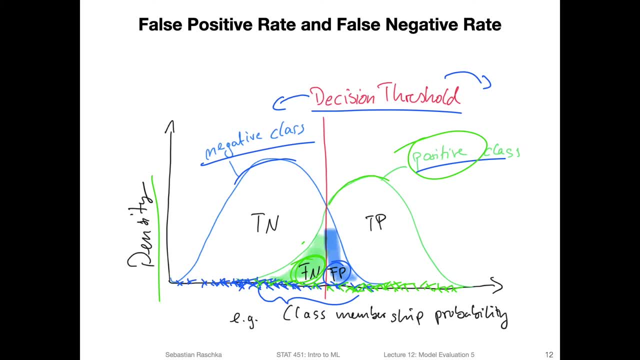 shift my decision threshold right So I could move it more to the left here. So if I move it more to the left I get more true positives right. So everything in this region now for the green one will be true, positive, So we increase. 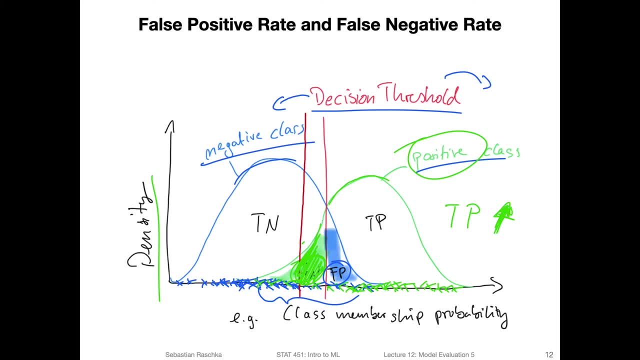 the number of true positives. just visualize by drawing an arrow up. However, at the same time, we also increase the number of false positives, right? Because now this one will be also now false positive. So we also increase the false positive. 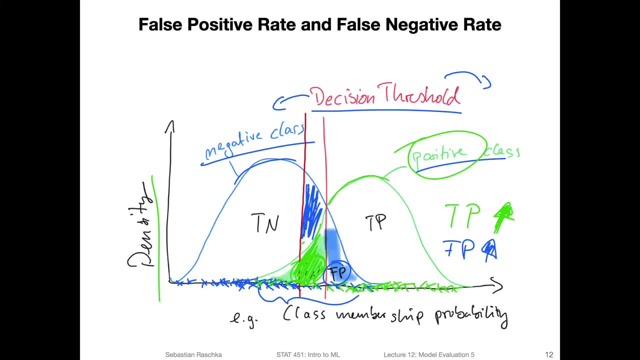 rate with that. So true positive and false positives go both up. And yeah, this is basically an issue: if we go the other direction, If I go here, we reduce the number of false positives, but we also reduce the number of true positives, So then we get a higher number of. 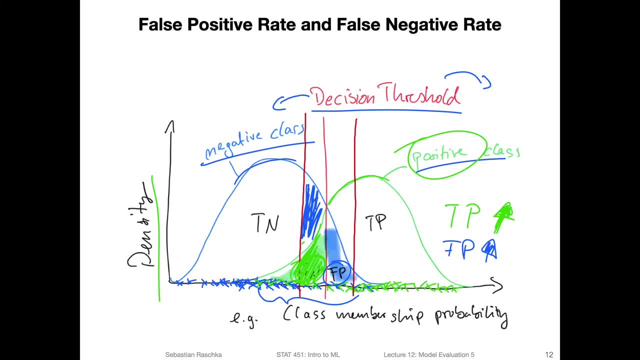 false negatives. So in that case there's always like a sweet spot between the two. So in this case a good spot would have been the original one, But depending on the application, maybe I want to reduce the number of false positives, So I 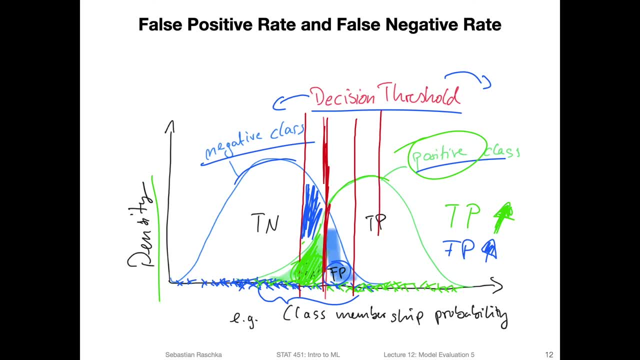 could, for example, in the spam classification example, try to get almost zero false positives and get fewer true positives. So I get more spam in my inbox, But then I avoid having important emails accidentally landing in my spam folder. So we will later in this lecture take a look at the 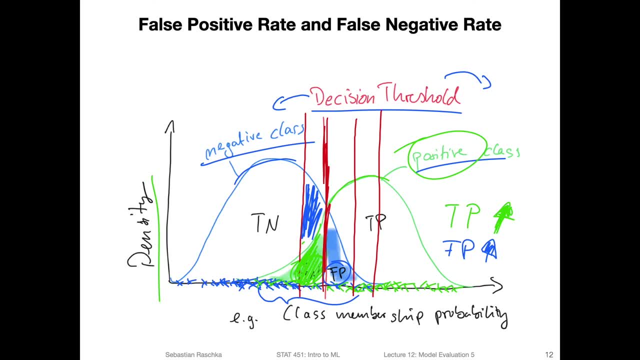 receiver operator characteristic, which plots the false positive rate and the true positive rate for different decision thresholds. So it's moving around the decision threshold and plots a curve where we have a true positive rate versus the false positive rate. And then we can, yeah, we. 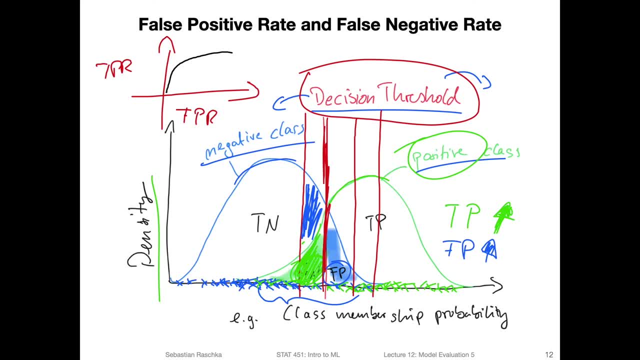 can then see how it looks like, And then we can compute the area under the curve, which can sometimes be helpful. if you don't have a particular threshold in mind and you want to compare different models to each other, then you can look at the models. 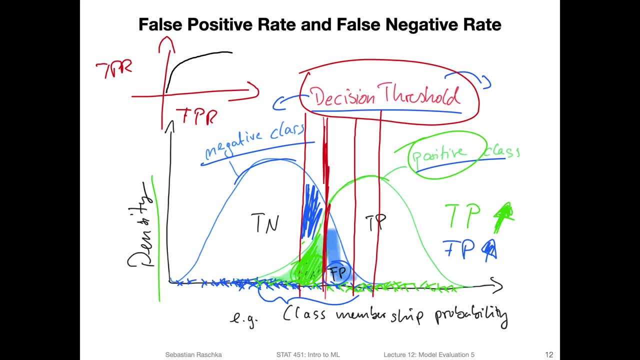 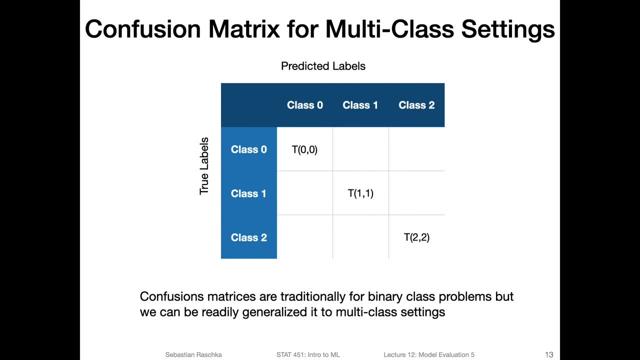 for different decision thresholds. It's also sometimes helpful to have a fairer comparison, but more about that later. So just to finish up the confusion matrix lecture here or video: Like I mentioned before, we can also construct confusion matrix matrices for more than two classes. So here I have a case.